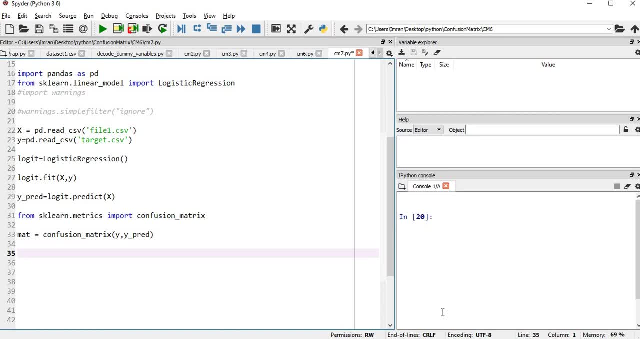 want to do it separately, if you want to do in one shot, how do we achieve that? what I will do: I will simply import pandas and I'll create a logistic regression model and then I this file one and target is my input file, the input variables, and also I have the target, like 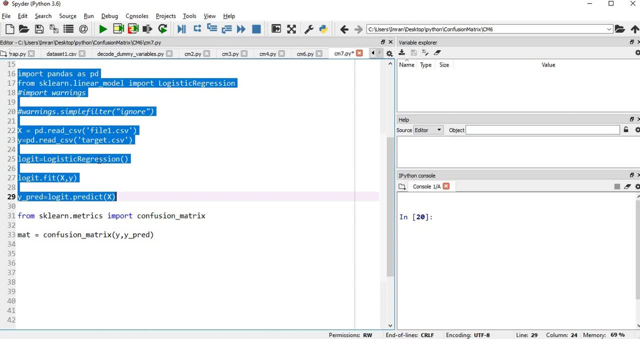 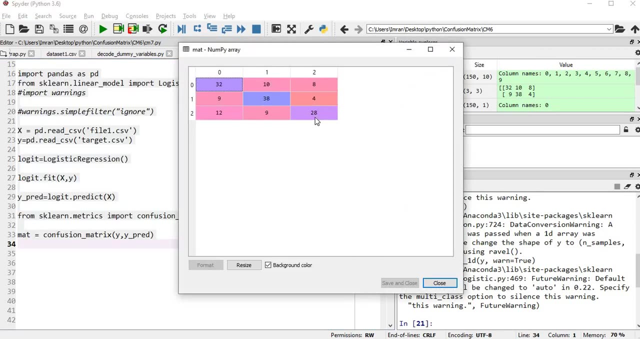 and then I'll create a logistic regression model. I'll fit the model and then I'll predict it. After that, I'll create a confusion matrix and then I'll create, I'll import the confusion matrix from sklearnmatrix and then I'll create a confusion matrix. so I'll execute this. okay, so this is exactly the same confusion matrix. 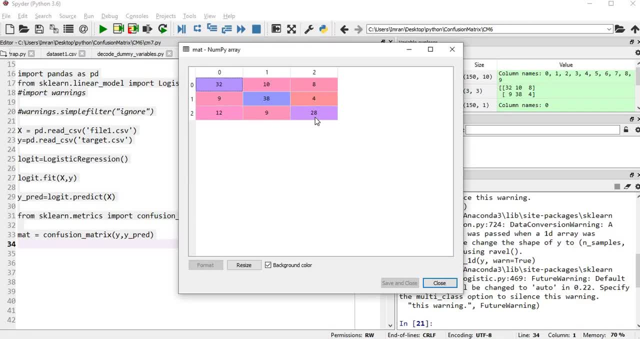 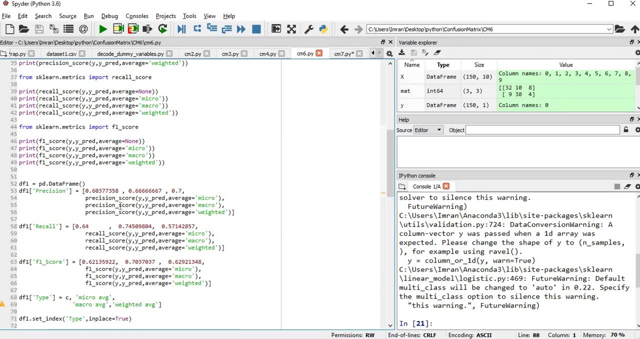 32, 10, 8, 9, 38, 4, 12, 9, 28. okay, now I have shown in my previous session, like how to get how individually, how we have calculated a precision score for micro, macro and for none, where individually it will come for all the classes, even for weighted precision score. recall underscore f1. 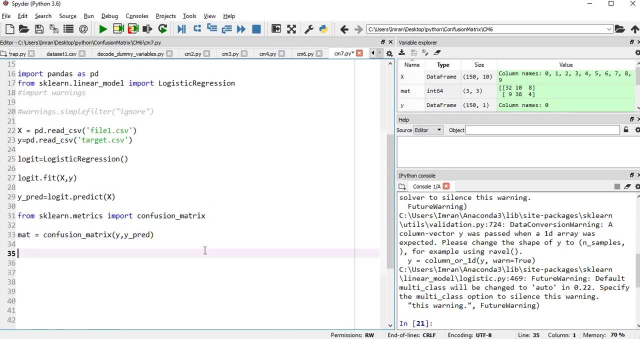 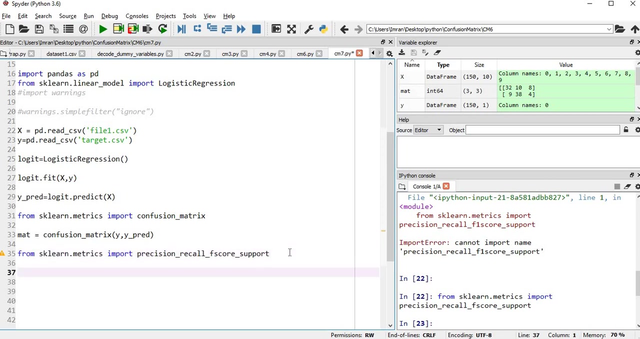 score everything. but I am not in favor of that. I want to save my time. so if we want to achieve that in a single shot, then we can. it can be done like this from sklearn import precision underscore. okay, this is my. this is a. I have written f1 square. it will be s okay now, simply, we can print. 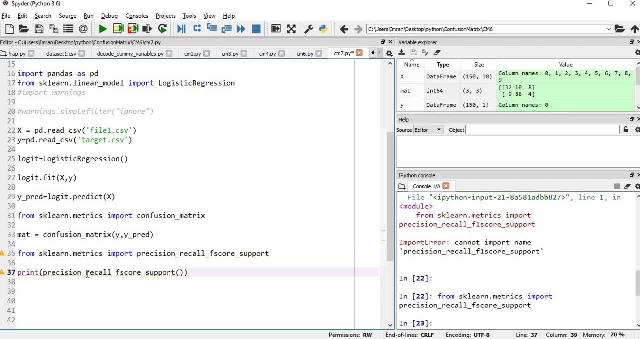 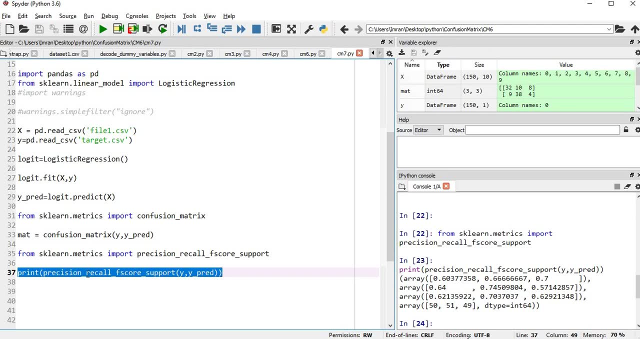 so I'll copy this and I'll paste it here and then I'll give the further score. So this is for a precision score, okay, but you can paste the variable, the particular value that you want under the y comma, y underscore read. so now, if this is the case, 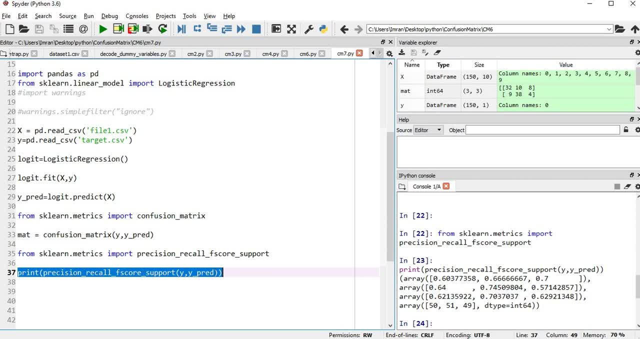 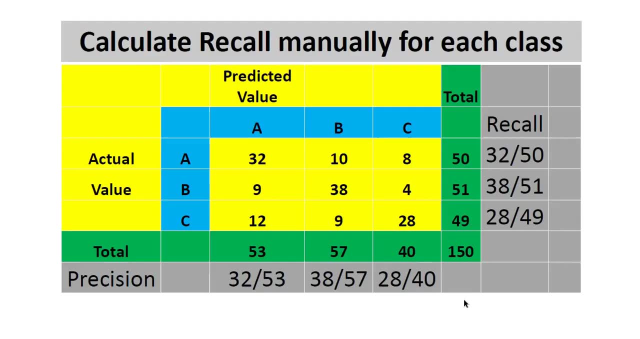 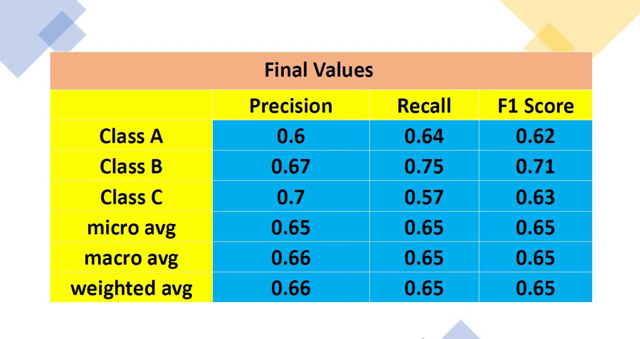 individually. the precision and recall will come, like when, if you don't pass in it value, it means none. so the first is the precision, second is recall: thirty s f1 score. now we we will come to our, we'll open our presentation and there we have the slide for our tabular format of precision. 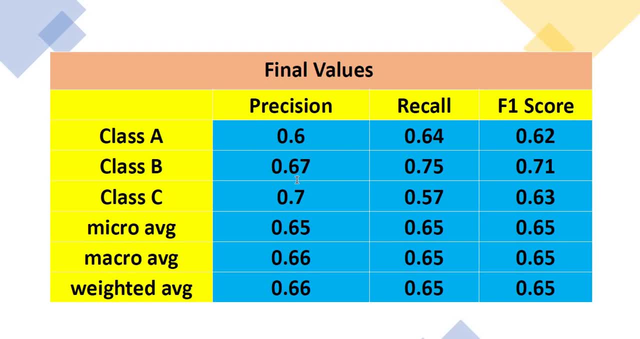 recall and f1 score. So if you see for precision for class a, Precision for class a, b and c are in the table here. if you see for precision for class a, precision for class a, b and c are in the table here is 0.6, 0.67, 0.7, 0.6, 0.65 and 0.7. for recall the value is 0.6 for 0.75, 0.57. recall the second. 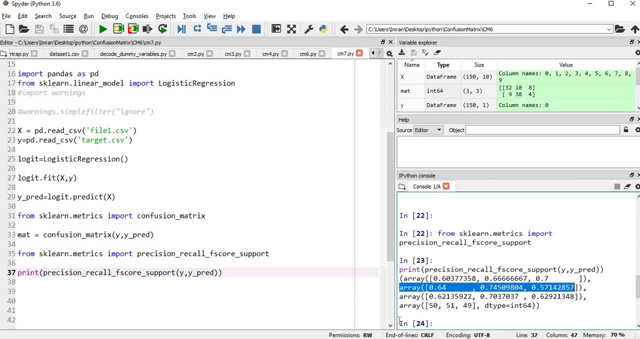 right you, we need to round it to the two places of the symbol. and the third uh row here is for f1 score: 0.62, 0.71, 0.63, 0.62, 0.71, 0.63. and the fourth one is the support is nothing, but if you. 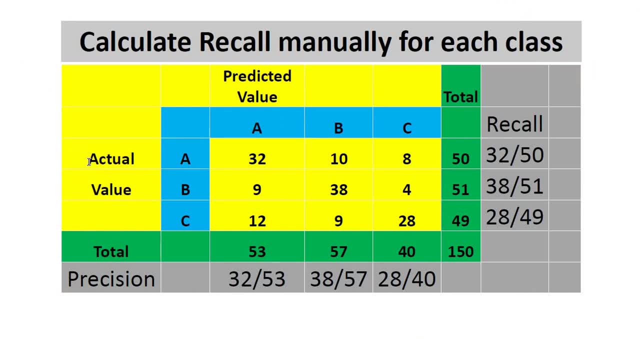 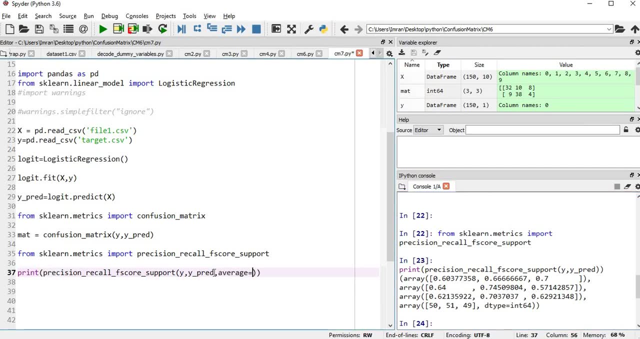 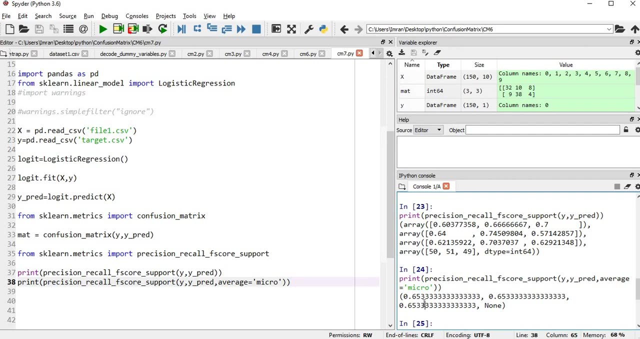 go here our total. total predicted like total instance of the actual value for each course. if we don't give anything, then it will assume. it will assume average to be none. if i want, average is equal to in that case in case of micro, okay, so what is my precision recall and f1 score? 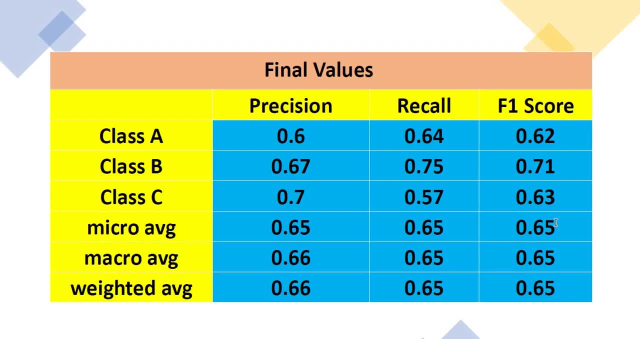 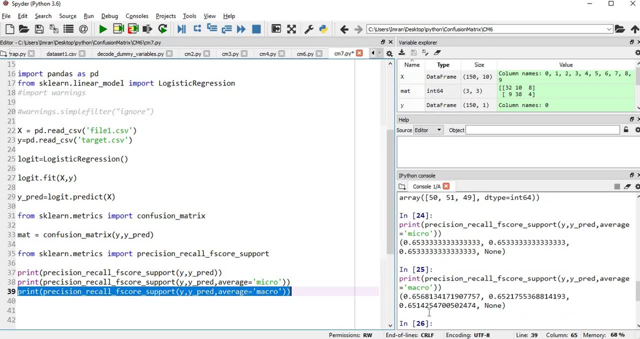 for k in case of micro, precision, recall and f1 score. all three of them are 0.65. all three of them are 0.65 right now. in case of macro, if i execute, this value is 0.66 if you round it to. 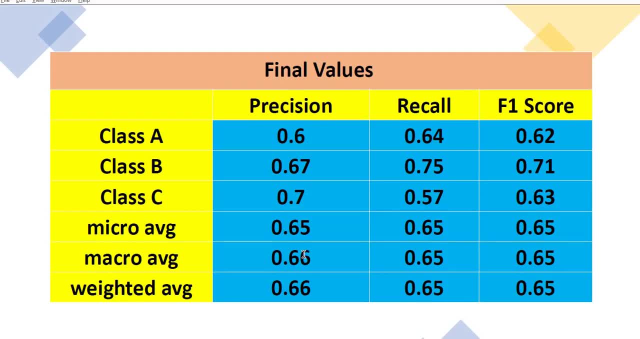 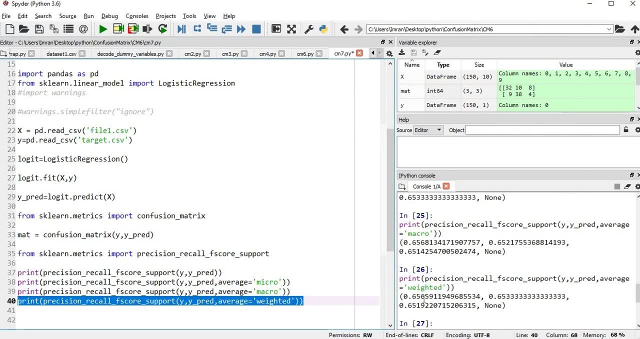 two places of the symbol, then 0.65, 0.65, 0.65, 0.65 and 0.65. now if we give here weighted, in case of weighted also it will be 0.66, 0.65 and 0.65. 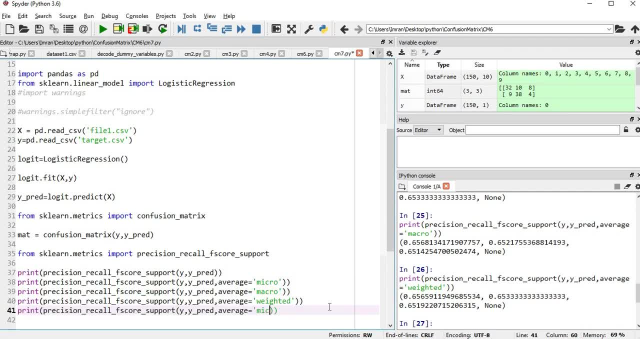 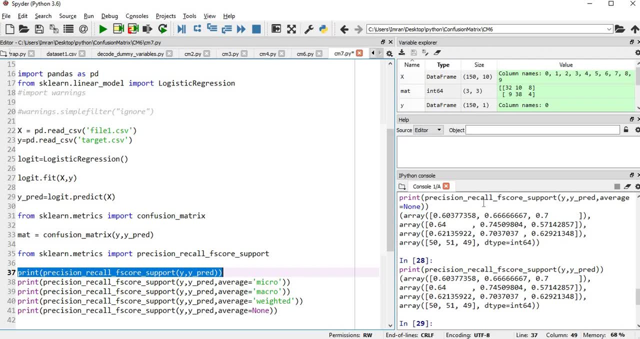 right. 0.66, 0.65 and 0.6, suppose i will say average is equal to none. average is equal to none will be same as if you don't pass the parameter by default. it will take this, so this is how we will use the. 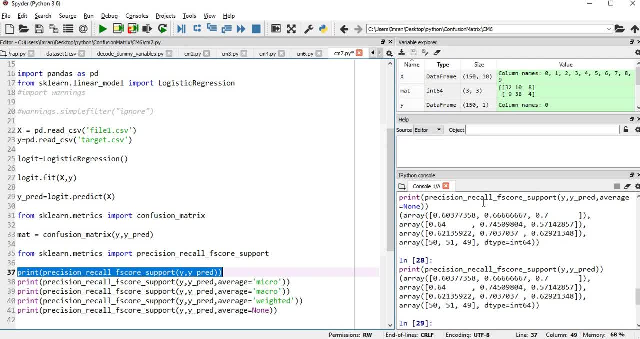 precision recall, uh score support from a scale and dot matrix and we can get the values for the precision recall and uh f score in a single shot. so i hope you like this video. if you liked it, please like this video. so thanks a lot for the uh for watching the session. this is one way of getting 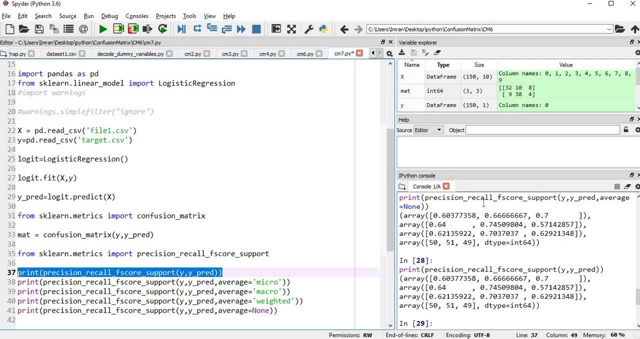 the precision recall and f score, f1 score. now in my next video i'll be showing you the classification report, okay, and also after that i'll be covering the pandas underscore: ml uh library. we need to import, so i'll be i am working on it and i'll be uh publishing my videos on a regular basis. 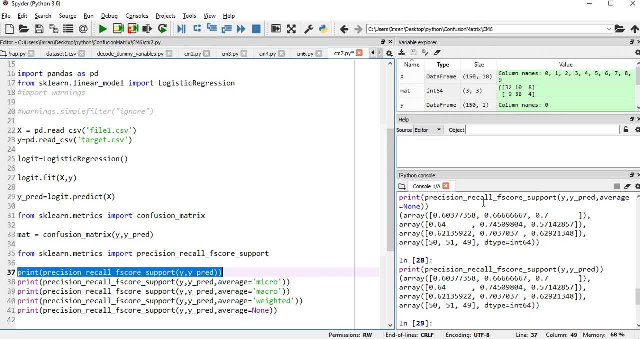 so thanks a lot for watching the session. if you feel this video is helpful, please press the like button and subscribe to this channel, and i will see you in the next video. thank you.